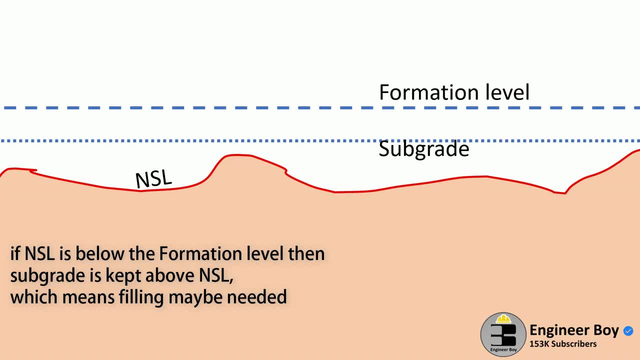 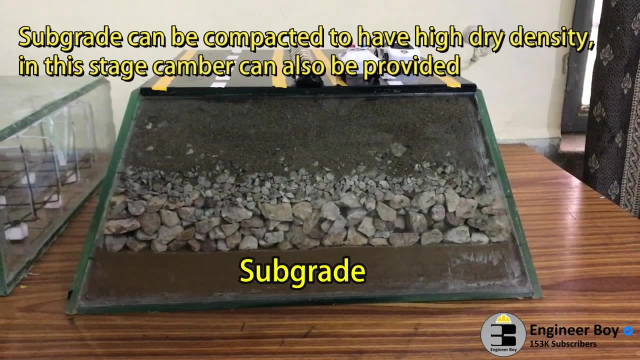 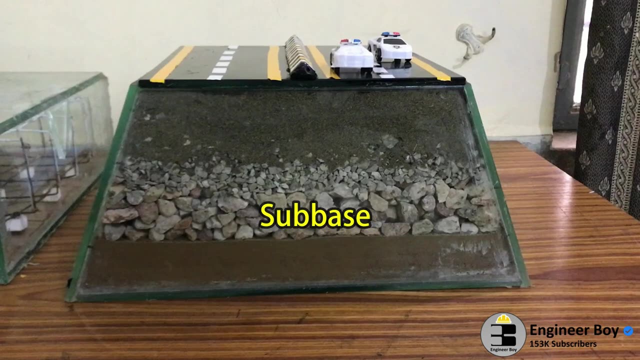 the formation level. then you can say the subgrade is kept above the ground level. subgrade is sometime compacted with ruler and camber. or you can say transfer slope is also provided to drain off the surface water. next we have sub base and of course this layer is just constructed above the subgrade. 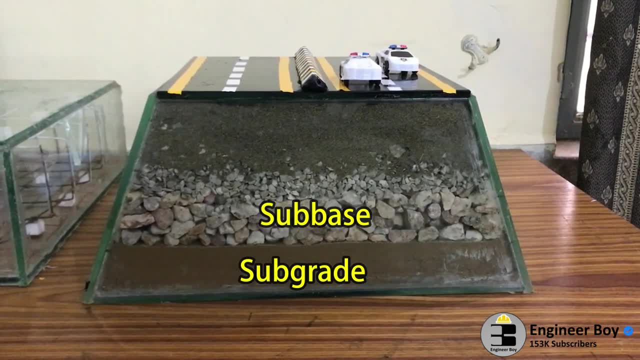 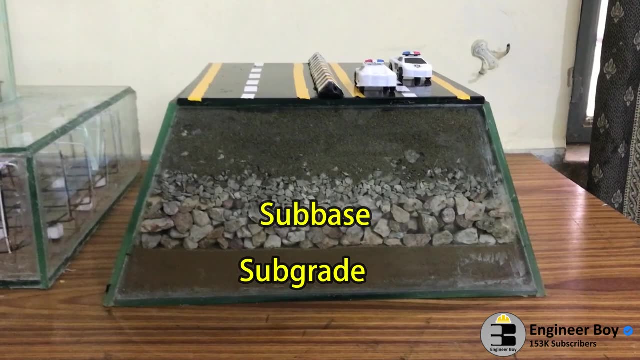 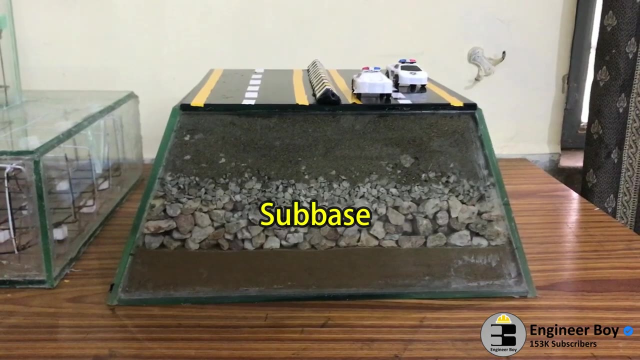 and if subgrade has high bearing capacity, then sub base may not be required. that means when you got subgrade with high bearing capacity, then there is no need to provide sub base layer. sub base is just provided to. or you can say prevent the rise of water, or you can say the. 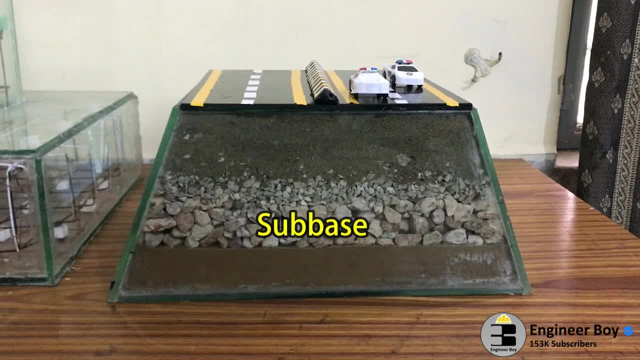 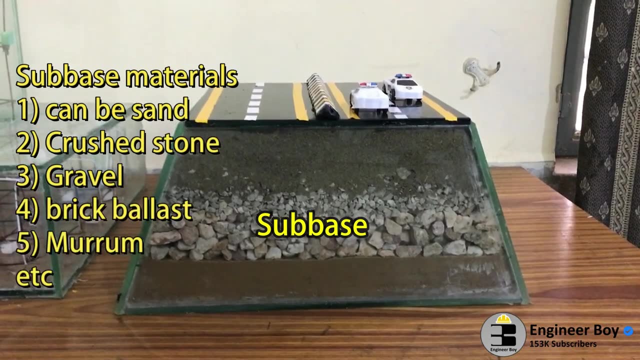 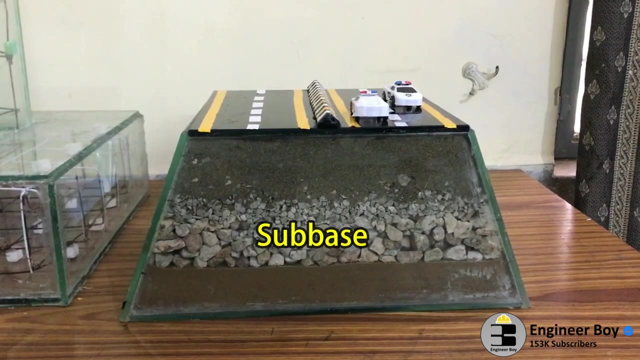 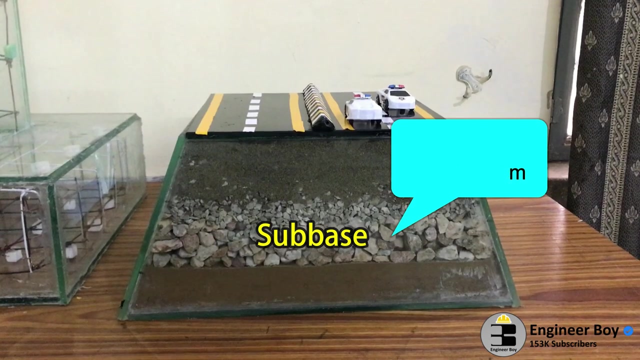 capillary action of subsurface water toward the pavement sub base can be just like the filling materials, or may contain the sand, gravel or sometimes stones. the thickness of this layer, or you can say the sub base layer, after compaction with eight to ten tons ruler, is normally kept at seven to fifteen centimeter, and then we have the base layer. 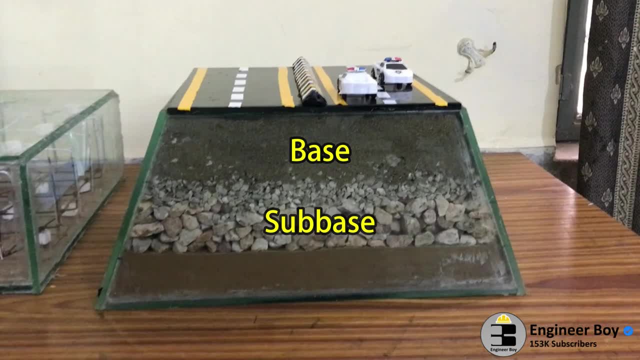 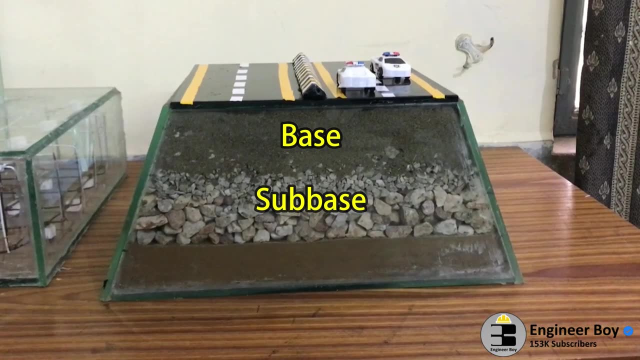 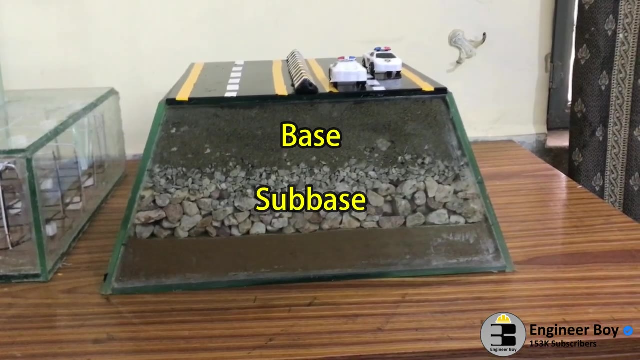 which is constructed above the sub base and it forms, like the foundation for the road surface or topping. this is just the main component of road which can be peeled of cement or maybe bitumenous concrete. the thickness of this layer depends upon the- uh, you can say the bearing capacity of subgrade. 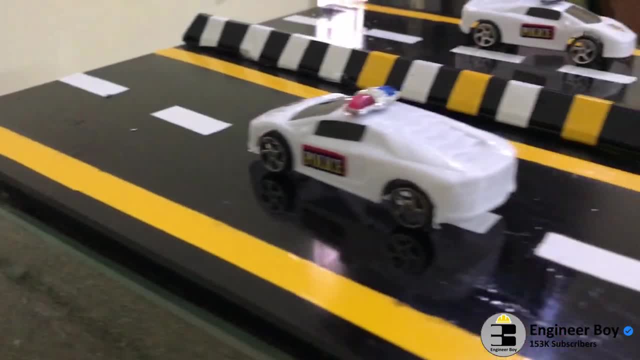 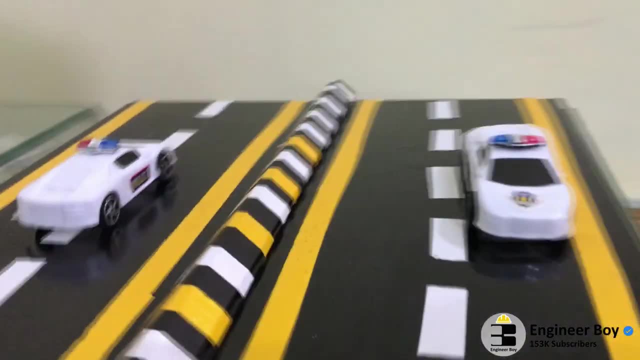 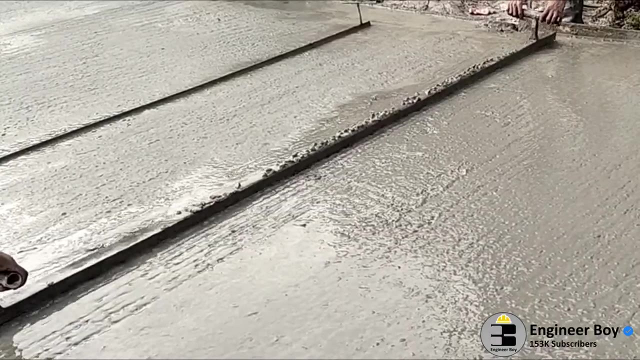 then the magnitude of the applied load and then, finally, we have the road surfacing or road topping, which can be, of course, made of bitumenous material, like for flexible pavement, as part concrete is used, and in case of rigid pavement, rcc or pcc may be used. this layer, i mean the the road surfacing. 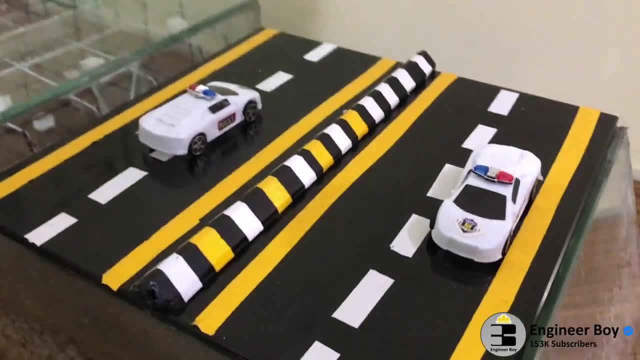 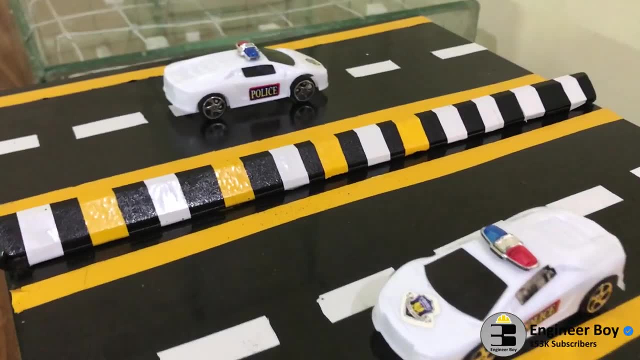 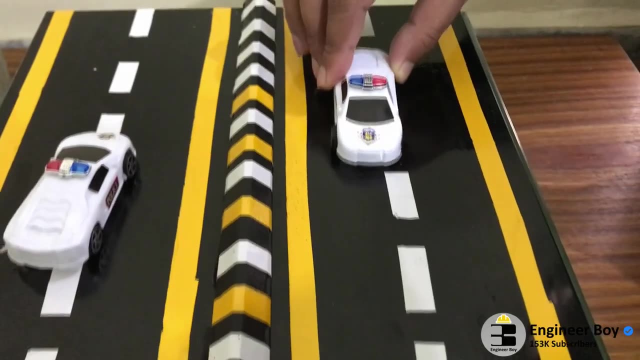 or you can say: the road topping prevents the penetration of water into the base layer and saves the lower layers from the abrasion and other weathering effects of the moving vehicle. this layer also provides smooth surface for the traffic, and that's it. this is what i got, and hey, if you like these types videos, please hit that. 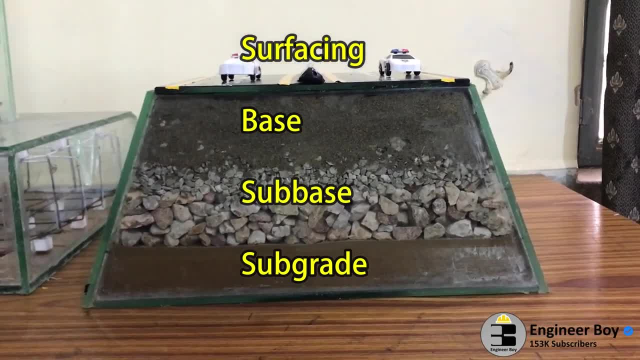 subscribe button. press the bell icon so you never miss an update from the engineer boy.